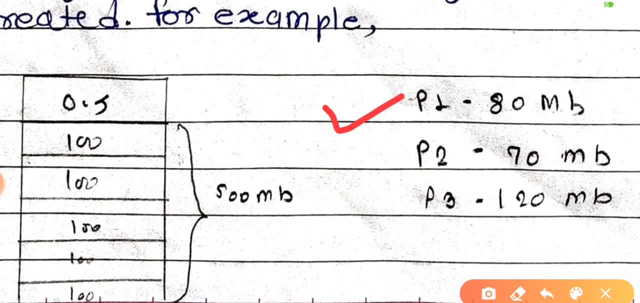 karthaedh dad size, i gmb tell up liquor. I say honey at the head. at TMB my giant she and this a video run car is I. then you will get this first memory. okay, memory space somebody. I process your requirement. I am CMB. 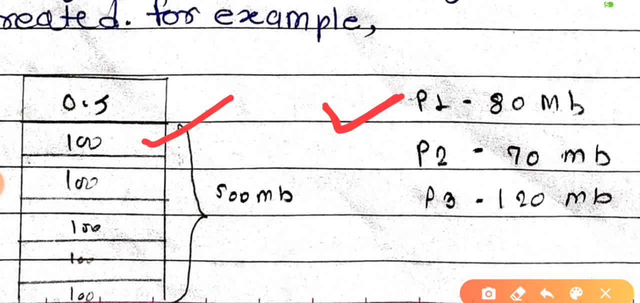 Kierton I, a ultra VCM be just a medallion, so it will easily run then. second, a process needs 70 MB. suppose this is another video. it will also get the relevant memory space. I can have more than requirement. better than easily, smoothly run home sale this reprocess, I suppose, as unequal a. 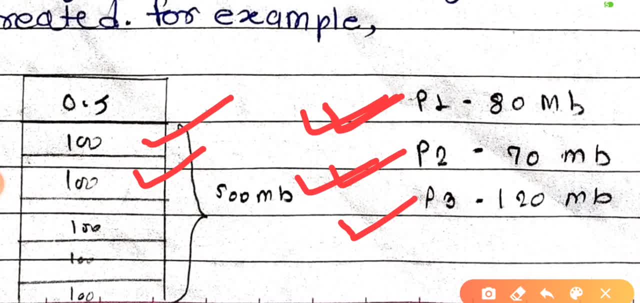 channel video song to me: run car that high quality I and that she sighs. I actually CMB at the. yeah, this area process la run on a sati. it a express recovery. I had a bug a to me. yes, I see some of the contiguous memory. 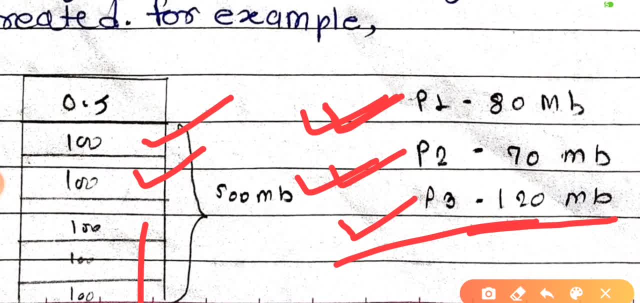 allocation after point, some of them with a malacca at the sale. you can see this is the first memory space and the second memory space is the first memory space and the second memory space and the second memory space. contiguous memory allocation. when Jekai the egg slug, a cut that you would ease. 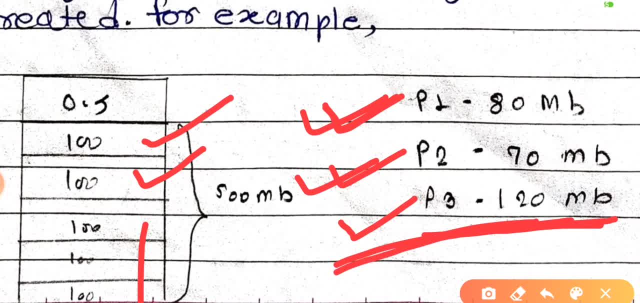 a guy available as me, the process la run on a sati. it a ektari saga a ghatta nahi a teriyala man top on fixed memory allocation. if it will be bogus akta fixed size memory allocation and he had a nook Sanka and if I deca. 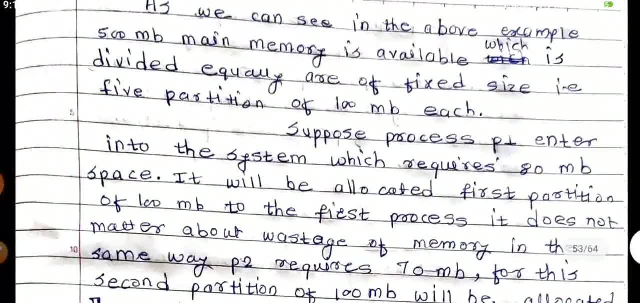 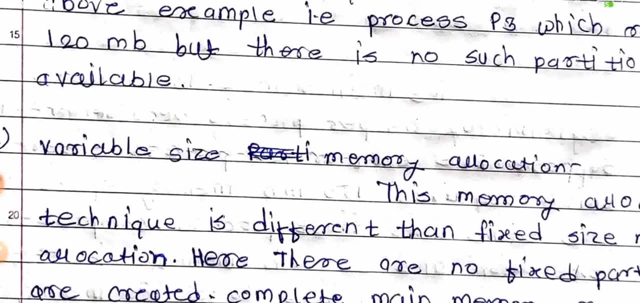 he said I'm just a mora, a ticket. Salah put a technique: the connoisseur Britain occur to need now but a variable size memory allocation. take a turn out is a tassel variable sized memory allocation. now at the chart I diagram the direct to malasam: June Sang Nasa, breath nakar. 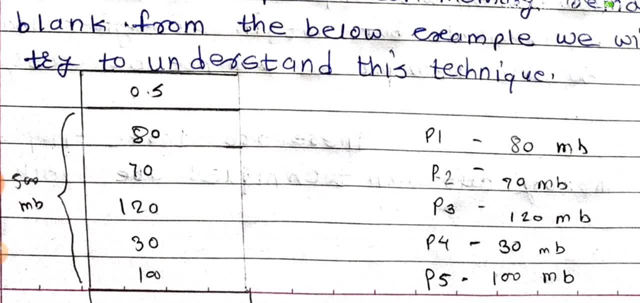 weapon, muda screen were bogus akta pass CMB dista, he passion be it. who need Paranthi passing in beach a plea memory? I'm in, Jerry, I'm ahead. yeah, mother, he partitioned perlet need bogus akta to me. pala acia head, usara sattra head and 312. 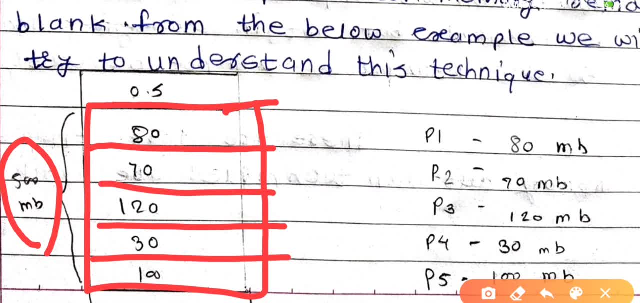 Isael and 30 sahib culture sombra: a randomly partitioned perlete. partition: randomly perlete panic cashier. issue: bonnipur, the talk you know, Contreras pattern, the product you're con Terec, while men, nosara, productive, excessive russie proceed, seal, tap, protect in a pattern of a per Sepata. 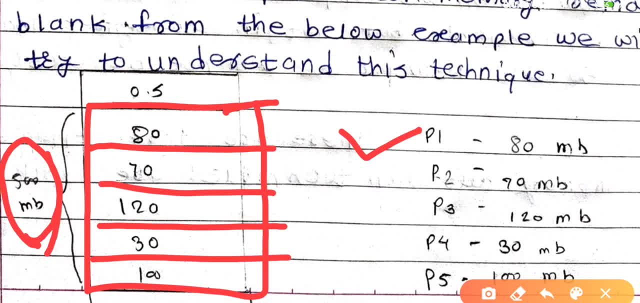 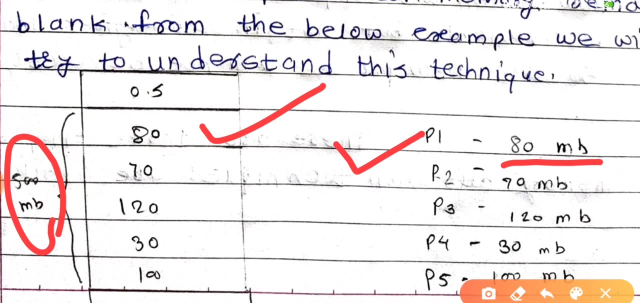 odournot established. a he eat ghatta the surroundings of passenger MB who the ticket some young a he's throughout a la passion be memory space. a he Polly process of the ledger requirement I. a 1st part is 80MB Available as per requirement. 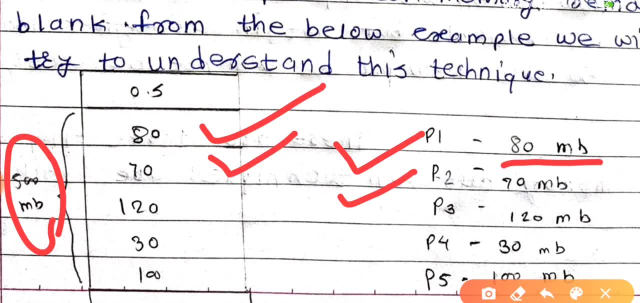 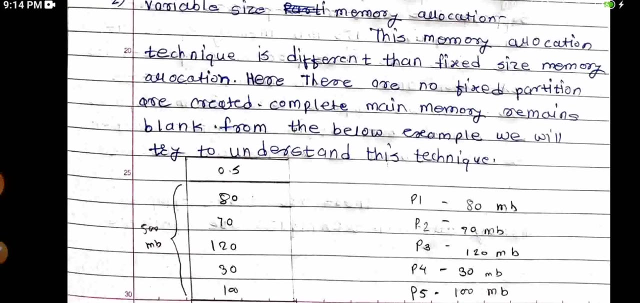 2nd process is 70MB. 3rd process is 120MB. 4th process is 30MB. 5th process is 100MB. 5th process is 100MB. All these are available as per required variable sized memory allocation. 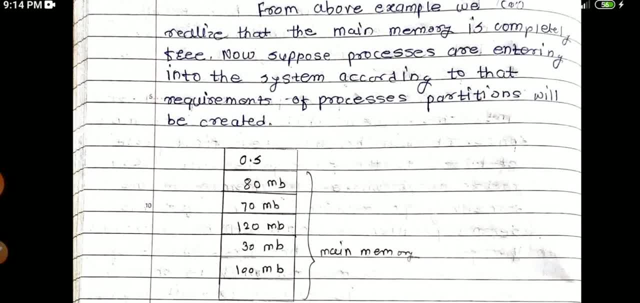 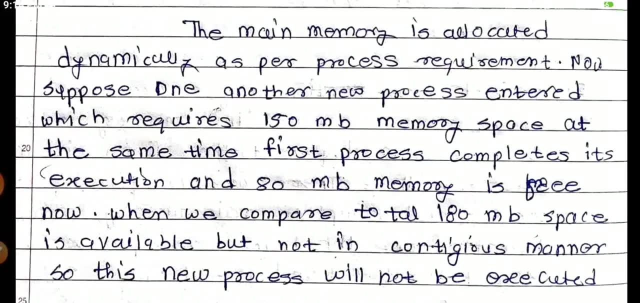 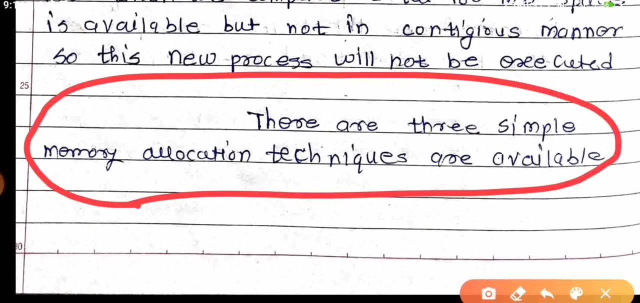 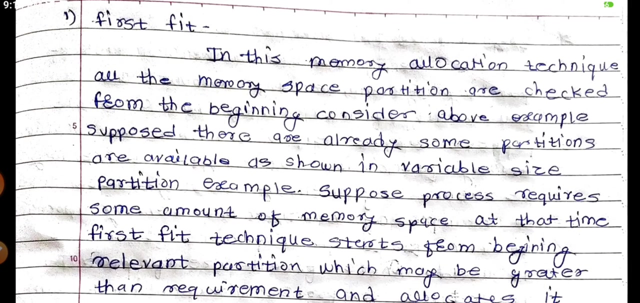 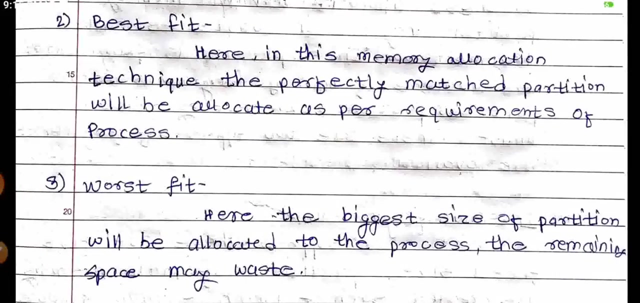 Now you have seen all the two main topics of memory allocation. There are 3 more important topics. There are 3 simple memory allocation techniques available, 3 techniques, 3 criteria: 1st is first fit, 2nd is best, 3rd is worst. What is first fit? 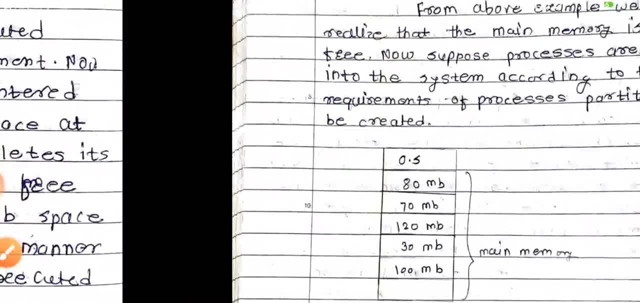 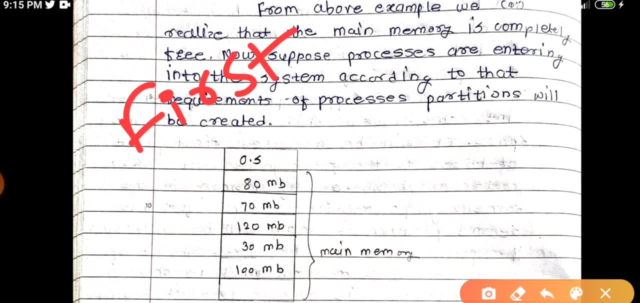 For example. I have shown you this diagram. This is memory. Let's see first fit, What is first fit. Let's see, There is one process P You have to check, For example, 100MB, 100MB, Is it in 1st check, 1st partition? 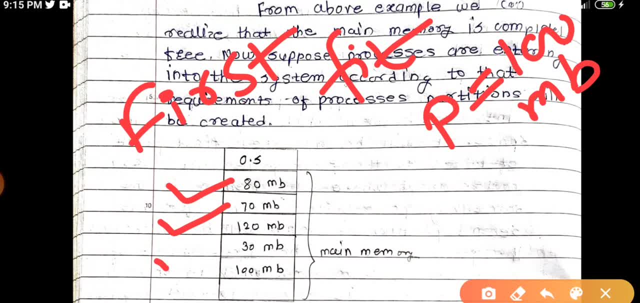 No 2nd, No 3rd: you have to check 100MB, But is available 120MB In this line. The space of 120MB will be allocated because it is the first row. If the first row is available, then the remaining 20MB will not be lost. 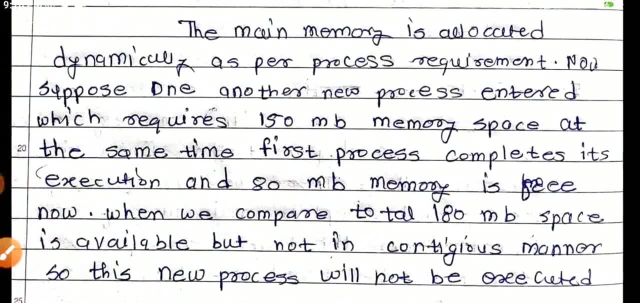 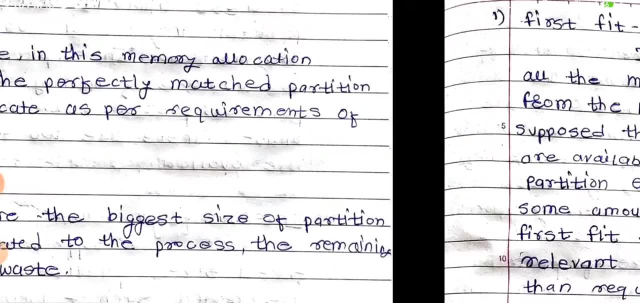 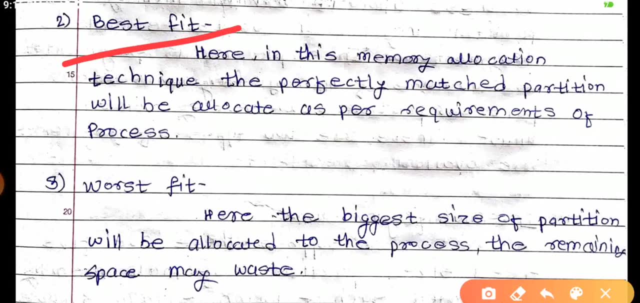 This is called the first fit, That is, to allocate according to the requirement in the line. The second type is the best fit. The name is the same: Best fit means to make the memory available as required And the third is the worst fit. 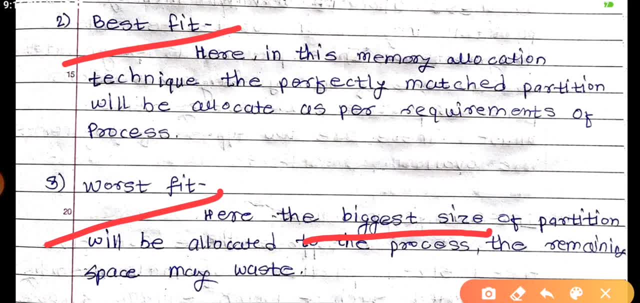 Worst fit means the biggest size, The biggest memory size or the highest memory size is available. For example, the requirement of the process is 100MB And one partition is 200MB And one partition is 240MB. If this is the highest piece, then this is allocated. 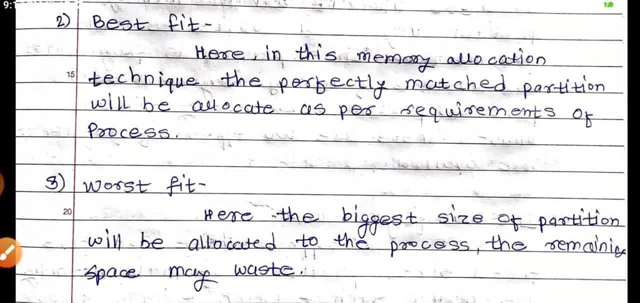 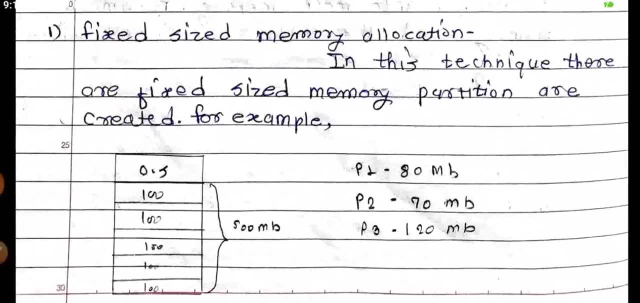 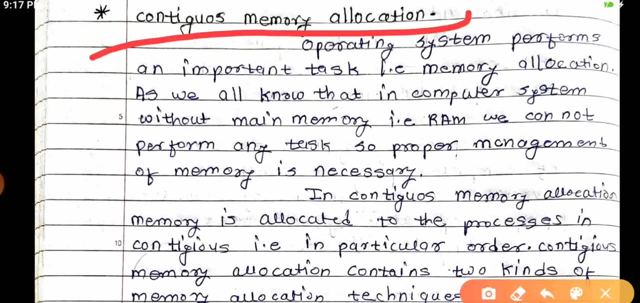 Then the remaining memory will not be lost. These are the three types. In this way, we have seen the issues of importance. How does all this come under? Let's see Contiguous memory allocation. Now we have seen the first point. 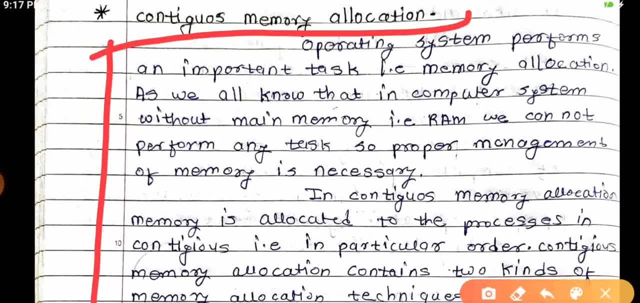 This is it. Everything is given in this. What I have explained now is that. Let's see once again what we have given here. Let's understand Contiguous memory. allocation means to make the memory available one by one. How, In the main memory? 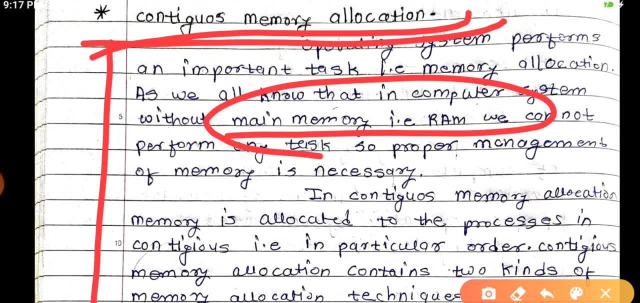 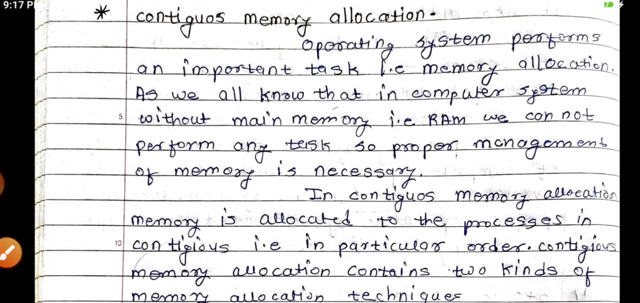 See clearly: Main memory means RAM. Nothing can be done except RAM. Without RAM, you cannot perform any single process. Simple, This is what is given here. Let's read it clearly. See: Not a single process can be performed. Cannot process. 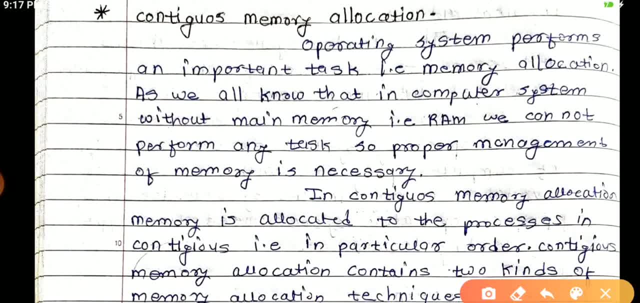 Okay, What is given next? See clearly In this contiguous memory allocation, That is, once a process enters your system, Any process in which you start in the system, in the computer. At that time it should be available as much memory as possible.